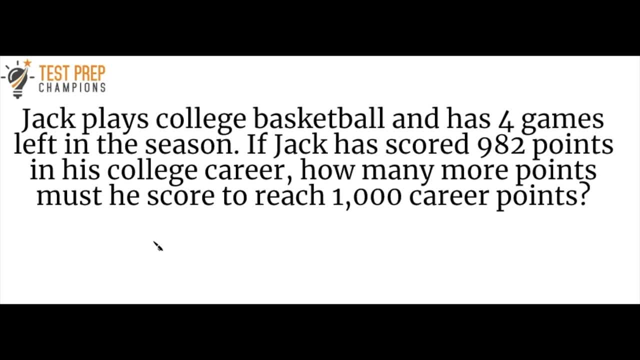 pause the video and try to do this on your own. Okay, so let's look at this. So we want to think of FIOS, and the F in FIOS is for find. What do we need to find? And so the last sentence really tells us what we need to find here. We need to find how many more? 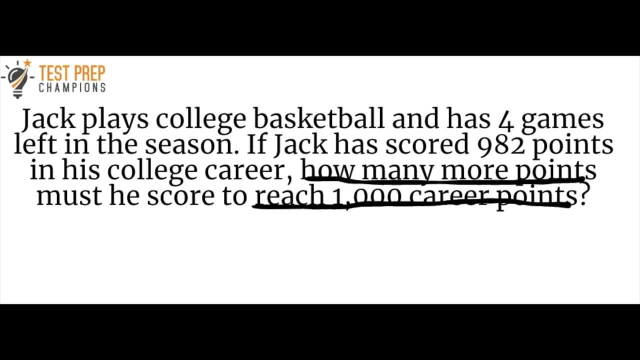 points Jack has to score to reach 1,000 career points. In other words, how many points are left for Jack until he gets to 1,000 points? So we've got the F in FIOS taken care of, So now let's move. 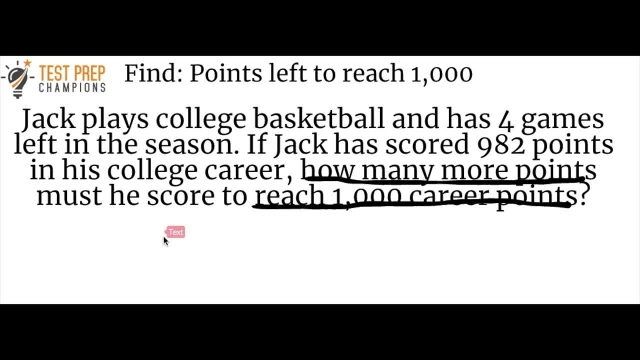 on to the I, which stands for info. Which information do we need to solve the question here? So the way you start is by looking at the info that you're given. So here we're given two different numbers. We were given four, which is for the four games left, and we're given 982 for. 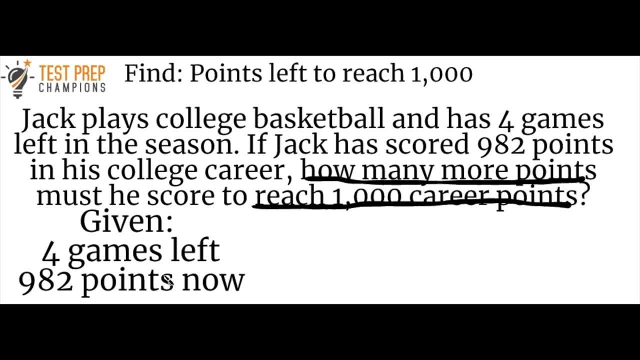 the points that Jack has right now in his career, And so what we wanted to solve here, remember, is how many points Jack has left to reach 1,000.. So we don't necessarily need to know how many games he has left, We just care about the points. Okay, so we've got our F and our. I done So now. 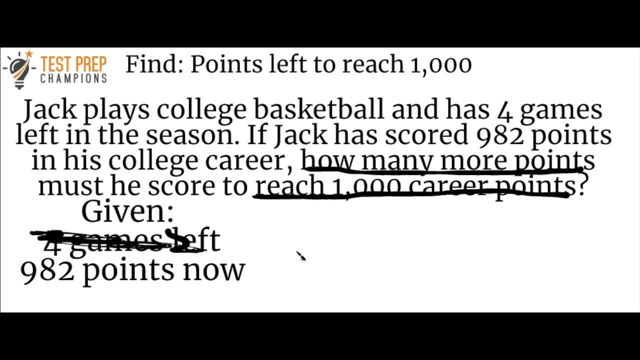 we want to look at the O, which is the operation, And we have to remember here that we're finding the difference between the 1,000 career points that Jack is about to reach and the 982 that he has now. So we're finding a difference. so that means that we're going to subtract here. So we 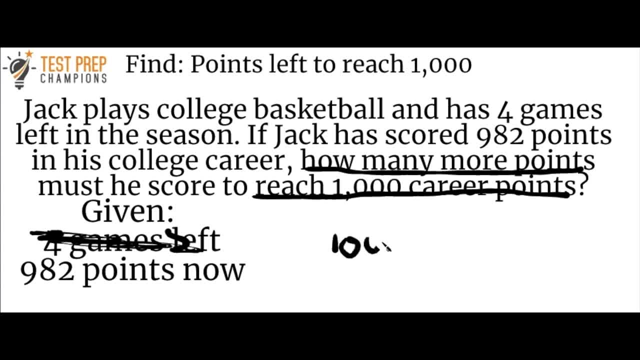 can set this up as a subtraction problem. So we've got our 1,000, and we are subtracting 982.. And the easiest way to do this, of course, is to just use a calculator, But we could also do it by: 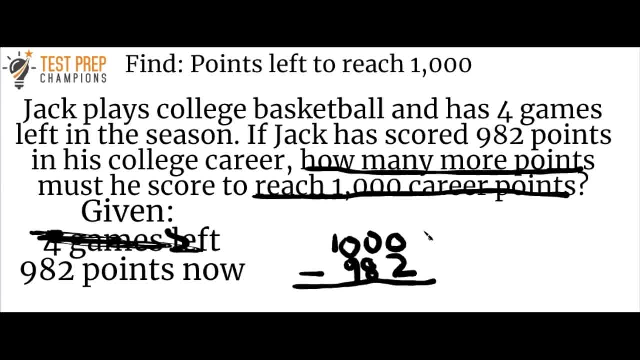 hand here. So let's do a little mini subtraction lesson here. So if we do 0 minus 2, we have to note here that 2 is a bigger number from 0. So what we want to do here is the 0 is going to look. 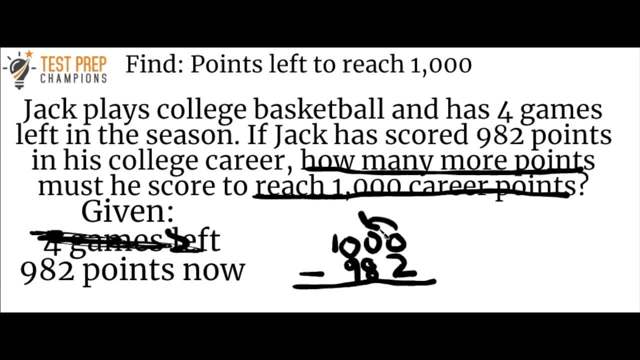 next door to the neighbor to see if the neighbor will let us borrow 1 here. And we can't do that here, So we have to go to the next neighbor and there's still nothing there to borrow. So we have to go all the way out to this 1, and we can borrow 1 here. So we're going to take 1 away from this 1,.